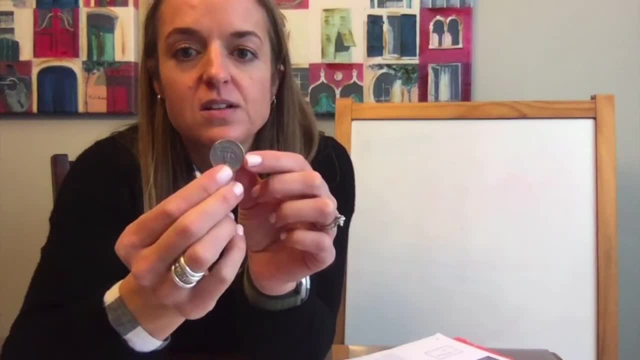 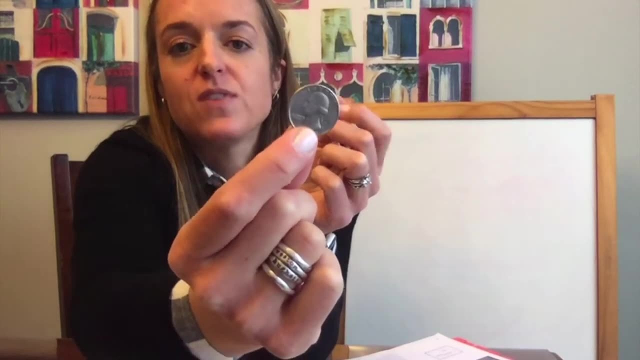 You see a coin has how many sides, Two sides. We usually call one the head's side, because there's an actual face on it. Most coins have the face of someone on one side And then the other side we call tails, and it might have any kind of picture on it. 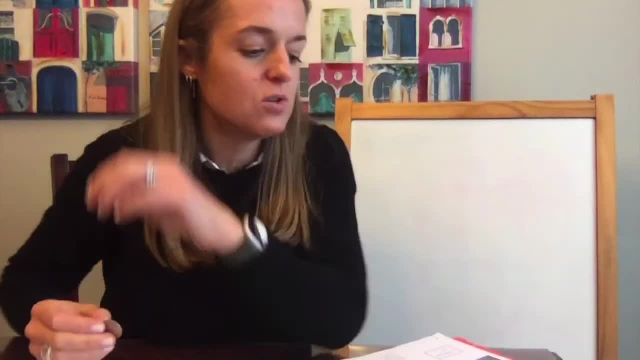 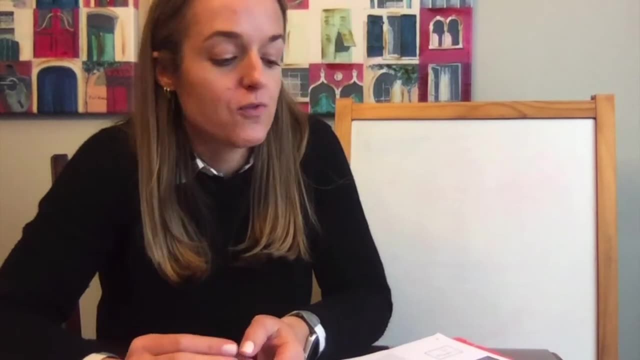 But we've got the head's side and we've got the tail's side, So two sides. If we wanted to play a game, one of the ways we could figure out who could go first or who can go first is by tossing a coin. 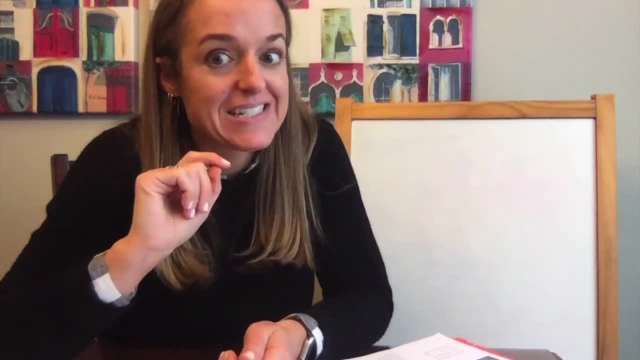 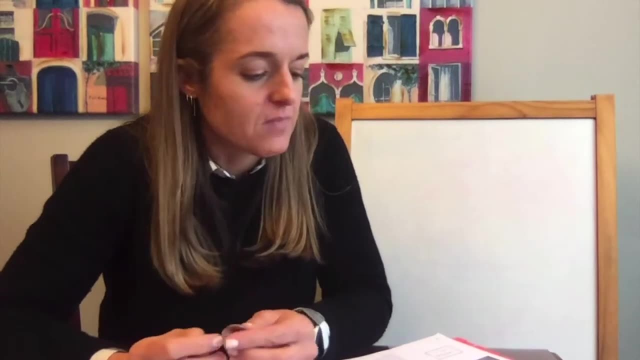 Can you think of a time when this actually happens in games? Yeah, like a referee might do it at the beginning of a football. I think about it with football: the coin toss and then they get to decide which side they start on, or whether they want to kick or receive. 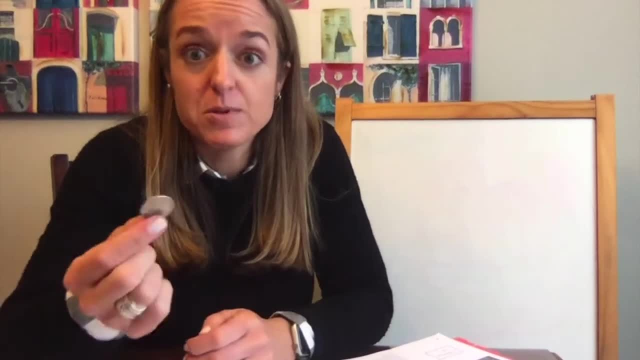 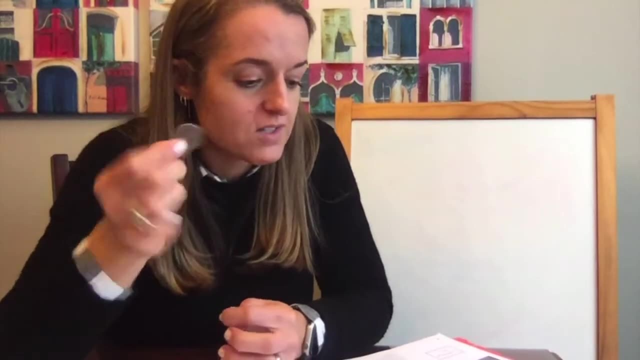 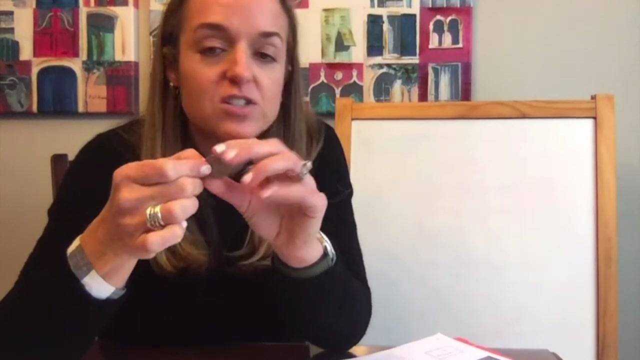 So the coin toss is supposed to be a fair way of deciding who goes first. Now, why is it fair? Why is a coin toss fair? Because there are two choices right, And there's an even chance of getting either heads or tails. 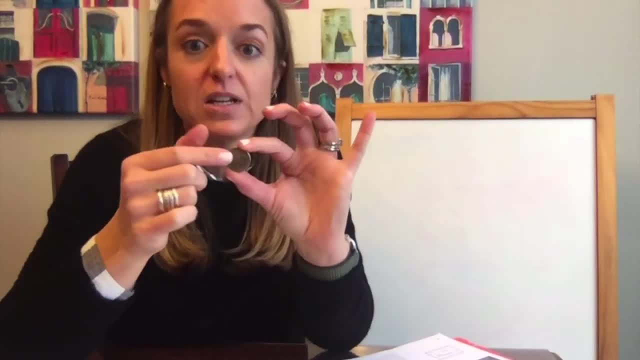 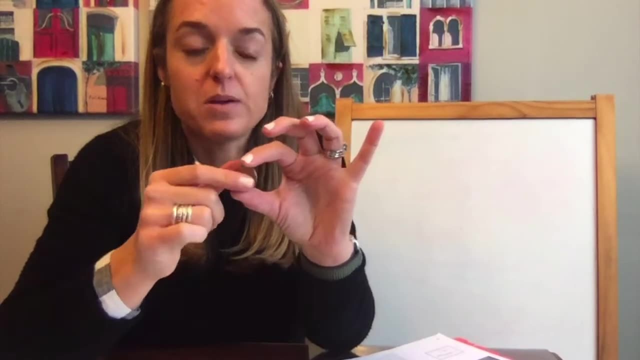 There's the same chance that you would get heads as that you would get tails. So that makes it fair. When there's just two choices, then this is a fair way of deciding which choice will be made. So we're going to test this ourselves to see if it's true. 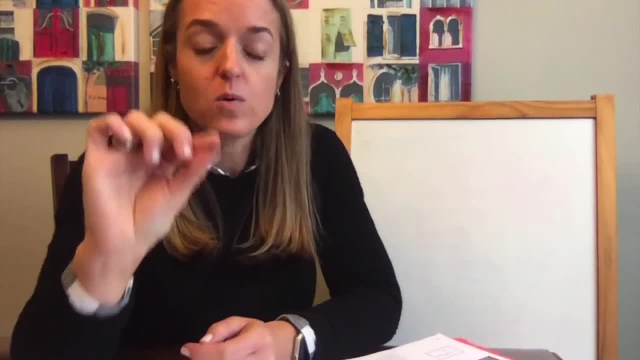 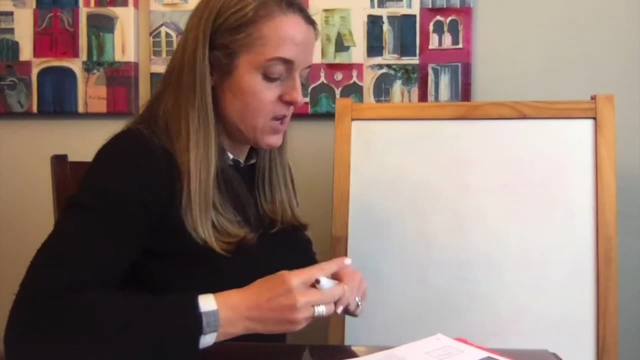 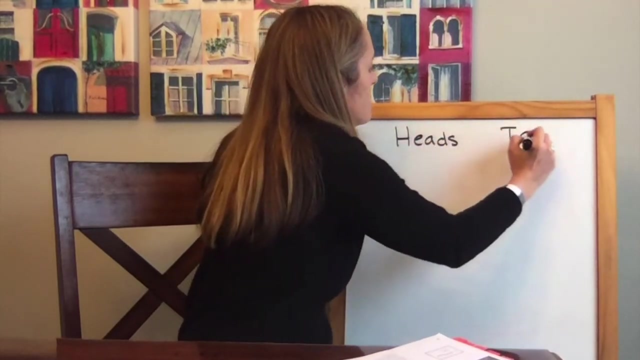 So we're going to work in pairs and we're going to flip coins, But first we're going to use paper and we're going to make a chart. All right, so we want to have heads, So we're going to have a ribbon at the top tails just to make a nice little T-chart here. 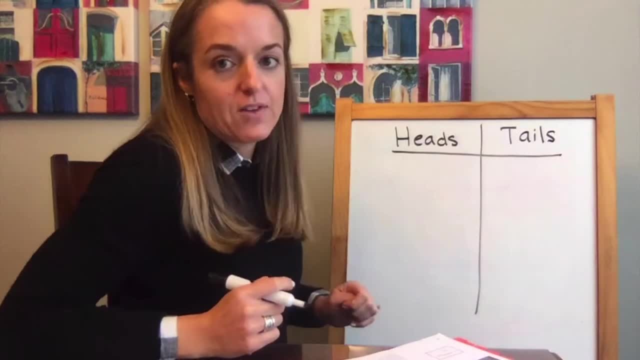 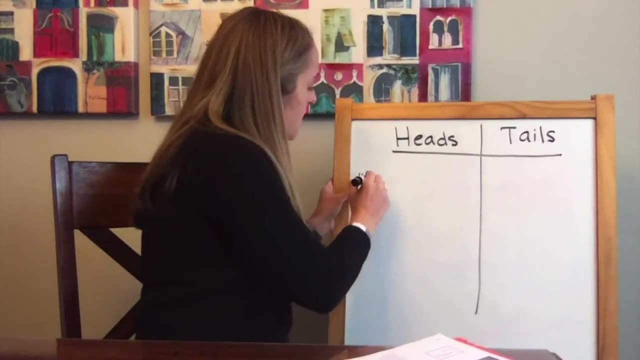 And then we are going to make tally marks to keep track of it. OK, so when we make tally marks, we're going to make that little like little ones almost, And when we get to number five we're actually going to cross through it. 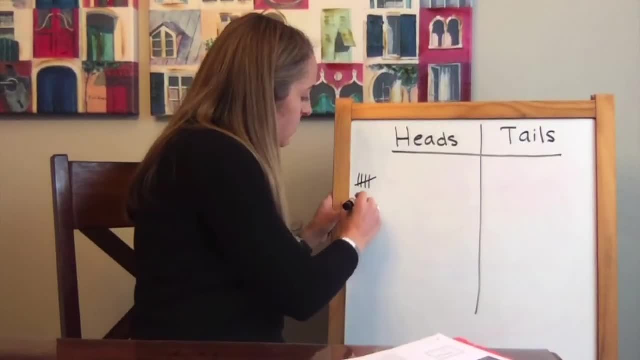 OK, so that's five, And then you start a new set. OK, and you can go side by side like this, If you want. The handy thing about making hash marks like this, or tally marks, is that when you're done, you can count by fives to count them. 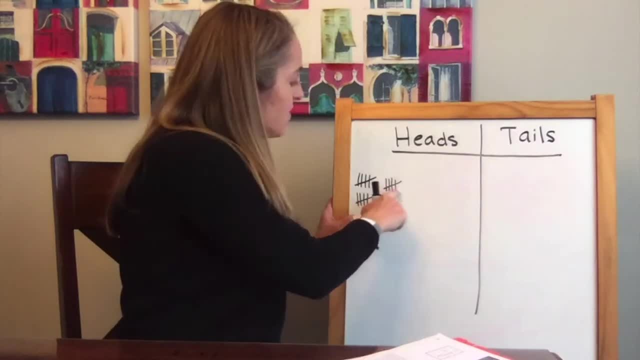 And we all know how to skip count by fives, right, Because we're in CC: 5,, 10,, 15,, 20.. And if I had a couple more: 5,, 10,, 15,, 20,, 21,, 22.. 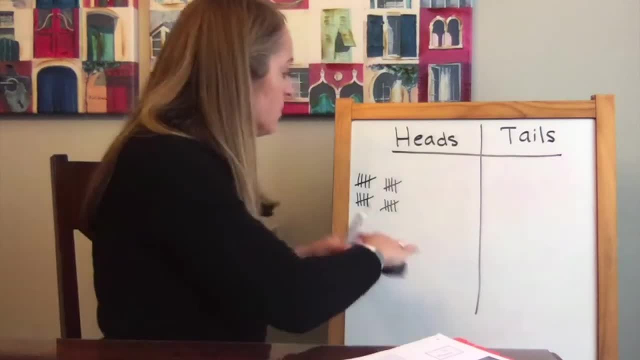 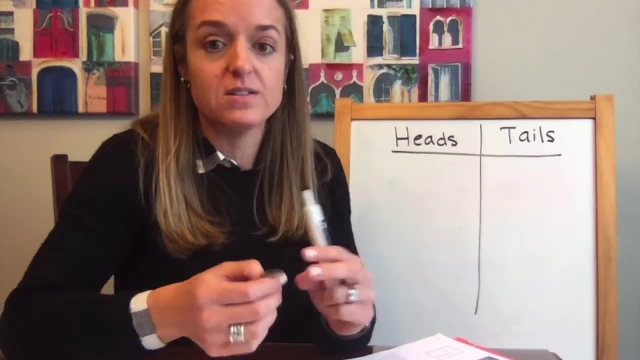 So it makes it really easy to count. So I think even our Obesavarians can do it that way. OK, so your pair, you guys have coins, And I want you guys to take two turns: flipping the coin and marking down. 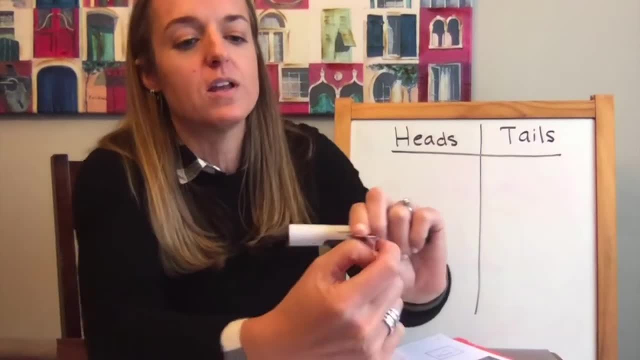 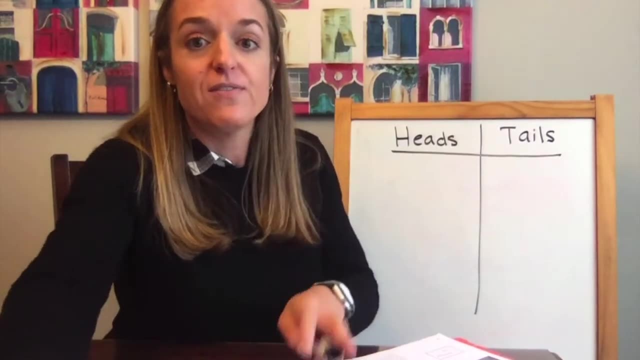 Is it heads or is it tails? OK, so the correct way to flip a coin is setting it on, kind of balancing it on your finger under a thumb and flipping it up. But if that's too challenging you can just hold it in your hand and kind of toss it and let it land on the tabletop. 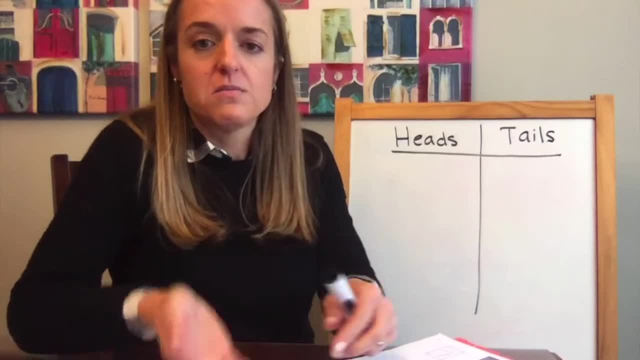 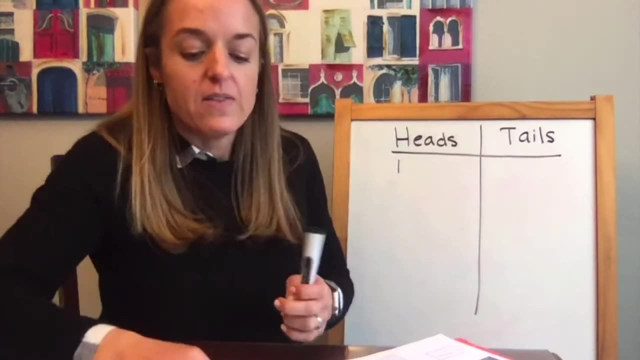 OK, we're not launching these across the room, We're just tossing them and seeing where they land. OK, so I got heads that time. So I'm going to make a little tally mark And then my partner can go. OK, and so then he's going to flip. 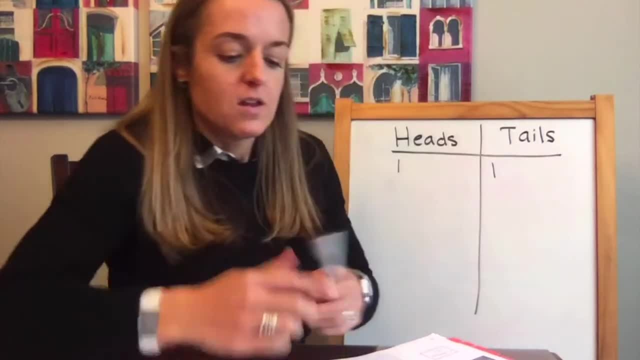 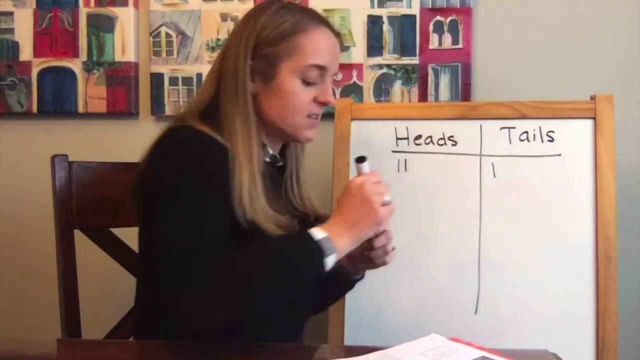 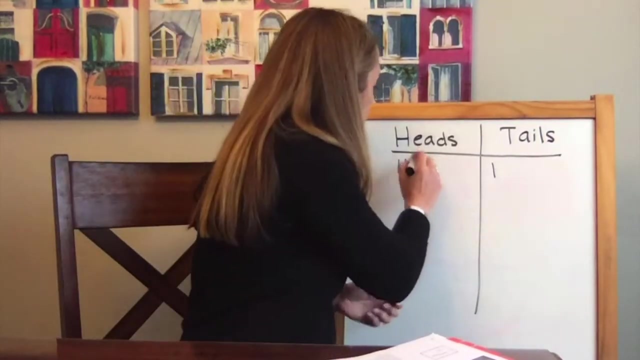 That time I got tails, And we're going to each do it six times, for a total of 12 tosses. Got a heads. that time I got another heads. OK, so you're going to do it 12 times. So let's pretend like we've done all 12 times. 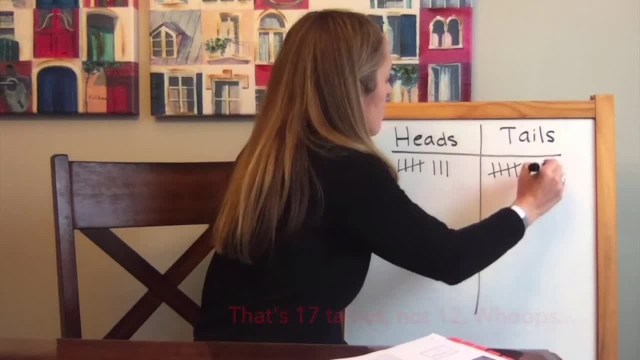 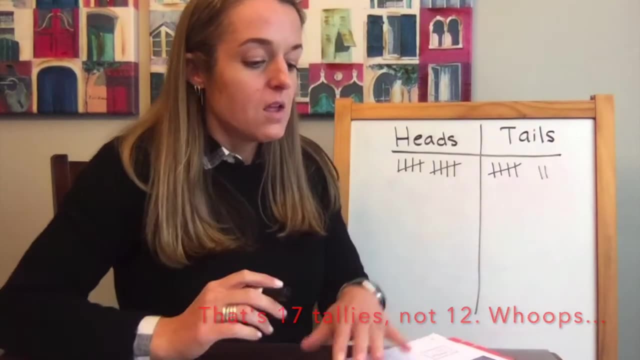 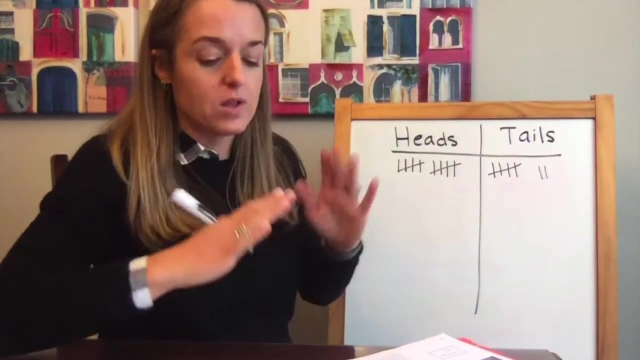 OK, let's just pretend like that's what we got. OK, let's just pretend like that's what we got. Now, once your part, you guys have gotten yours, then as a class, you guys can add up how much the whole class got OK. 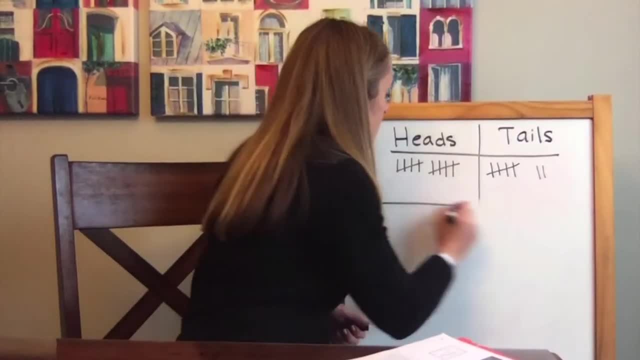 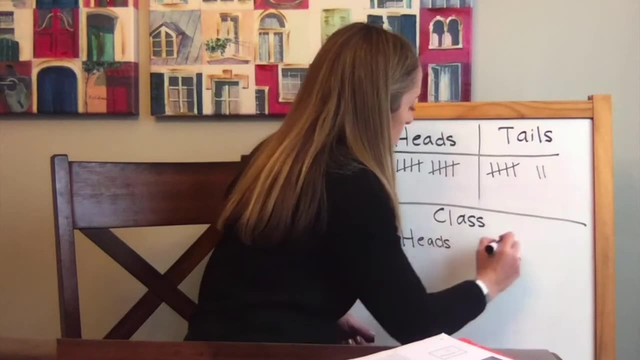 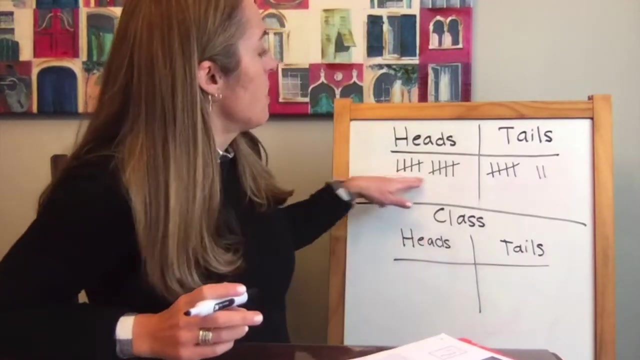 So your tutor might draw something Class. you might draw this on the board, something very similar, But it just shows the heads and tails of the class. So if we say we got ten heads because five, ten, right, Five, ten, We got ten heads. 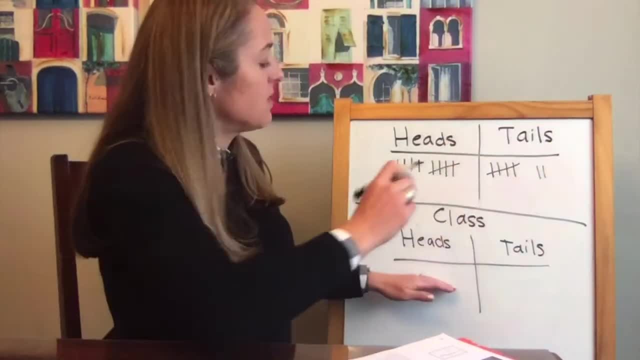 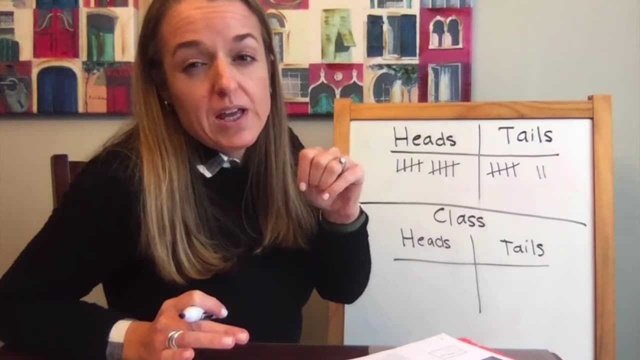 And that pair over there got eight heads. Whatever we get, let's say if we have four pairs in the class and we did 12 each, that would be 48 tosses, Right? So let's say we got twenty five heads. 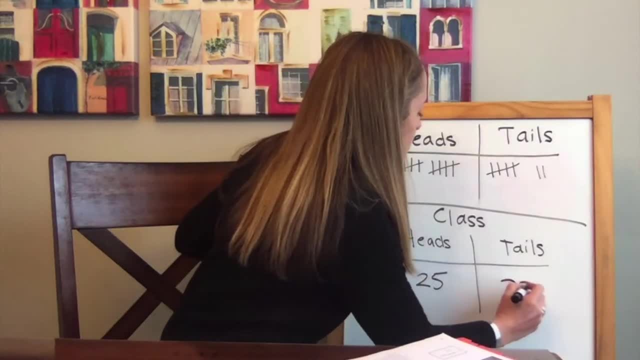 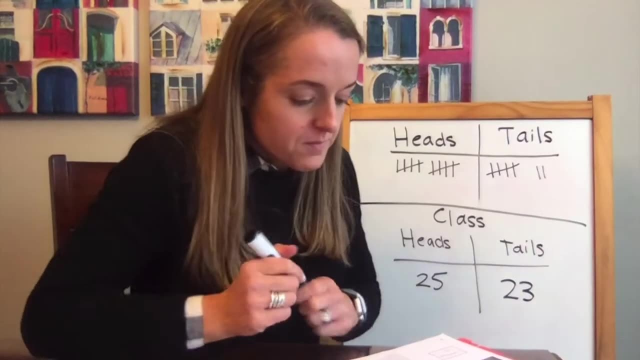 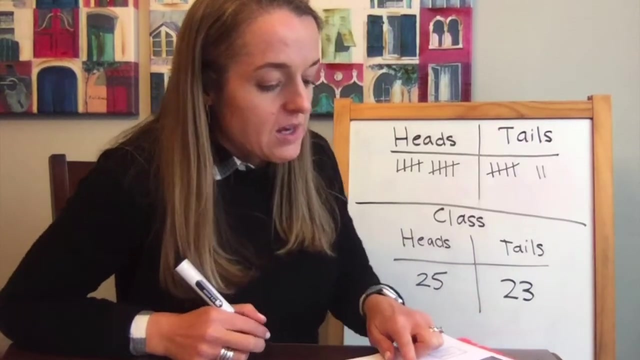 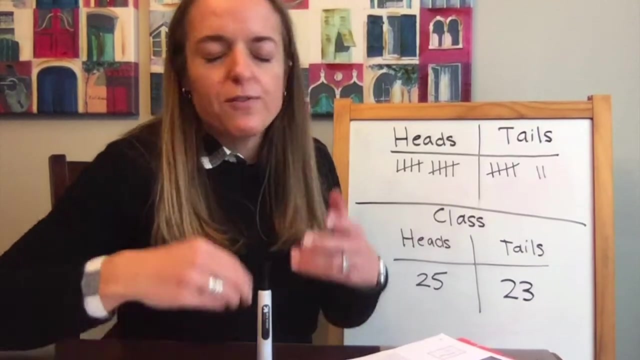 And Twenty three tails. So that is our class total. So that's our class total that we summed up to get our class results. now, If your coin landed on heads, Do it for sure. land on tails the next time, since that's the other choice. 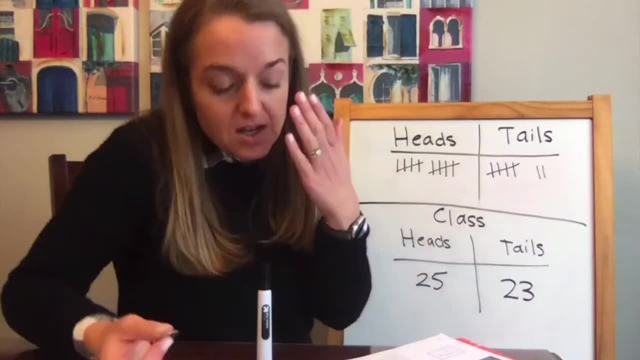 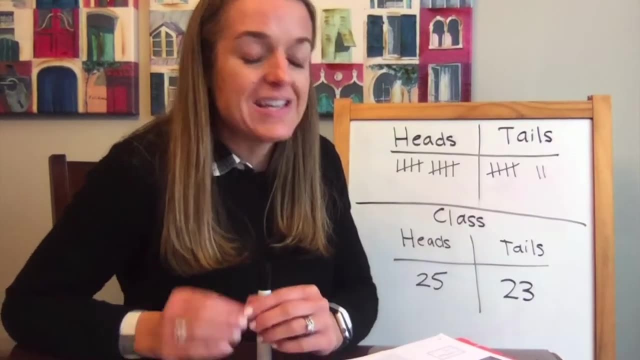 does it always go heads, tails, heads, tails, heads, tails. Does it do that? No, because we all understand that every flip of the coin is independent, and that is why we are. we are usually happy to use a coin to get a chance outcome. 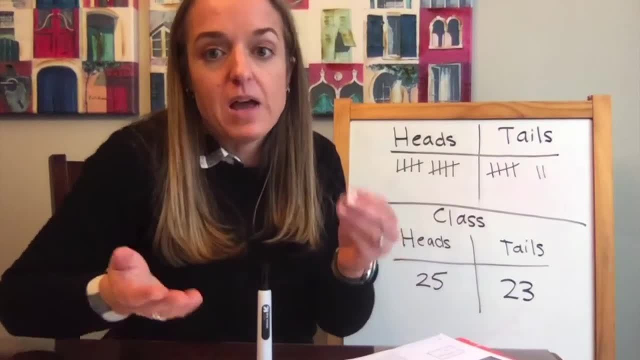 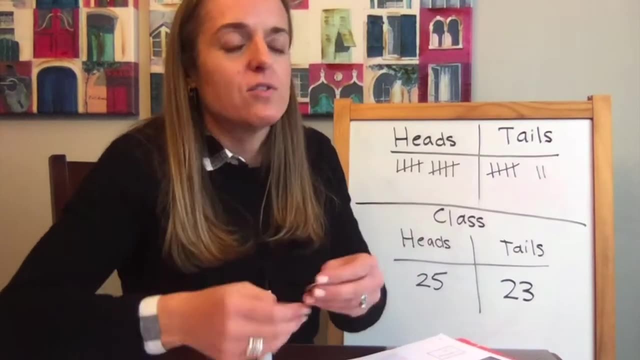 If we knew it was going to be every other one, every other one, that wouldn't really actually be fair, because you would just know: well, I want the second flip, because that's the one that I am asking for, or whatever. So you know that each flip is all by itself. 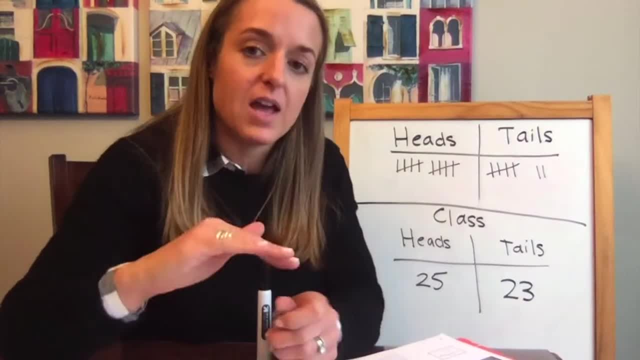 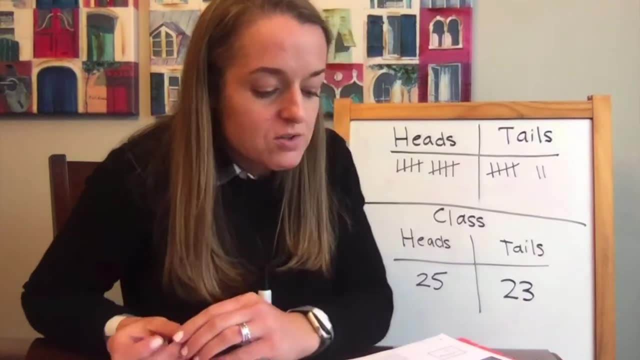 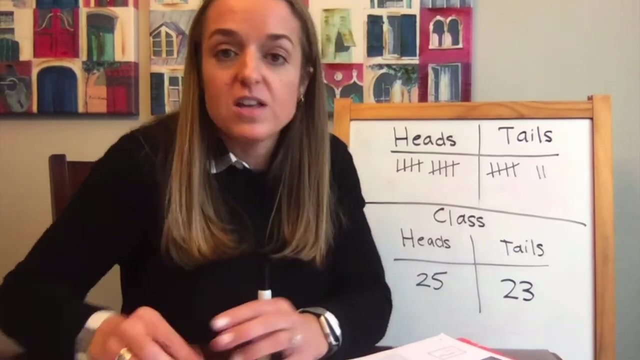 It has the same chance every time you flip it, of either being heads or tails. So that's what makes it fair. The mathematical study of this chance is called probability, And each time we flip the coin, our result is called the outcome. OK, so we've just learned the word independent. 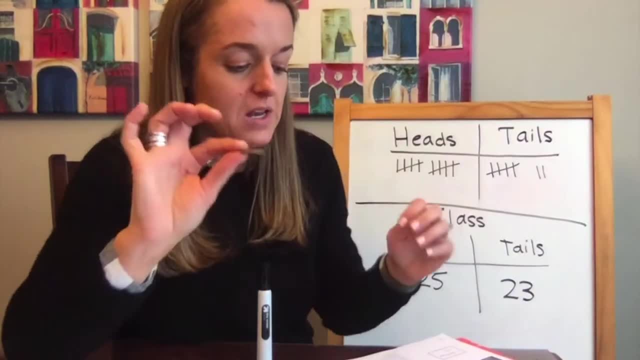 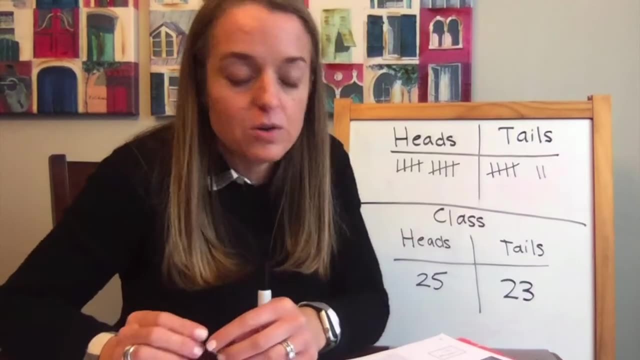 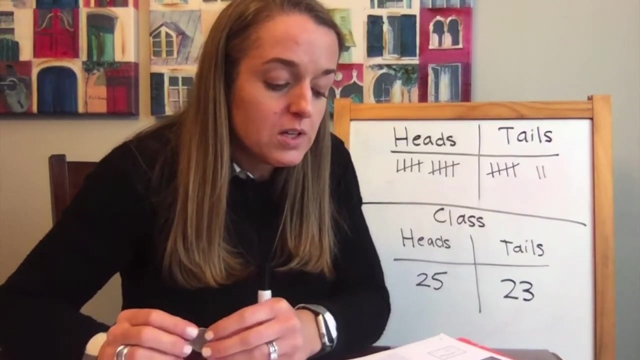 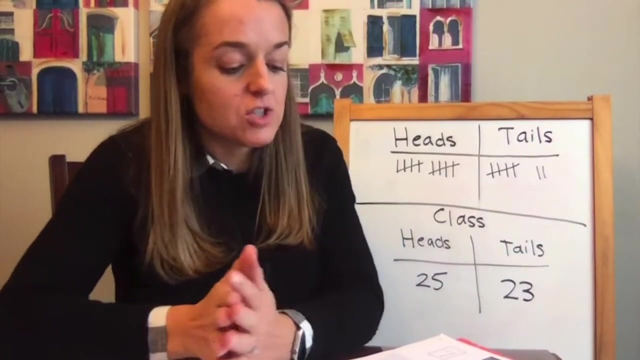 which means each coin toss is independent, the result is independent, And the study of this is called probability. And each time we flip the coin, our result is outcome. In the study of probability, we generally refer to desired outcomes, which are the outcomes we want or are interested in, and also then the total. 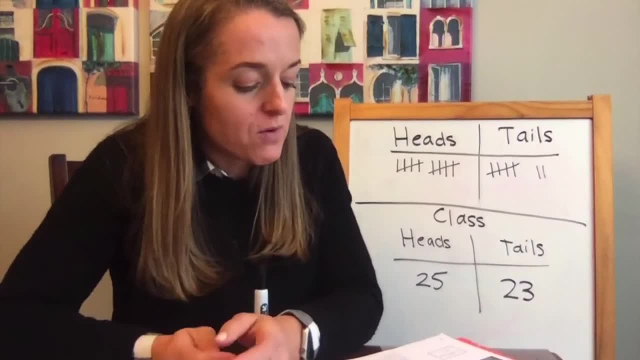 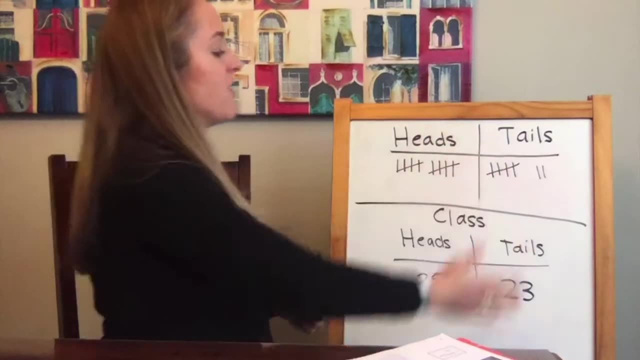 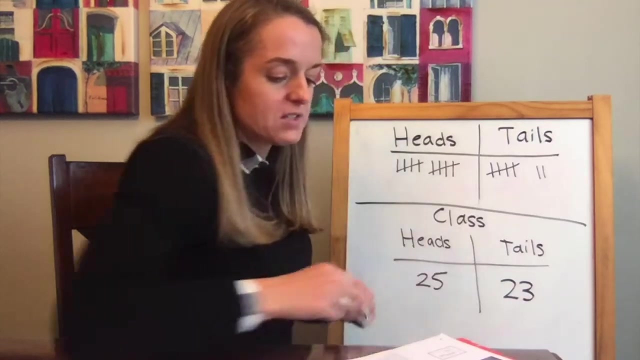 outcomes, which is everything that happened. So we may refer to events which mean an outcome or group of outcomes. So the event of us as a class flipping the coins is our twenty five heads and twenty three tails. That's our event. But and then our outcome? 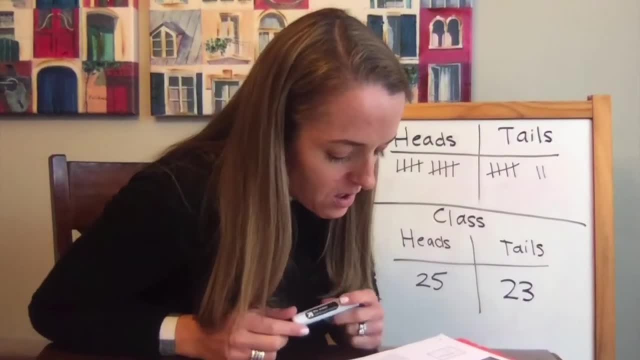 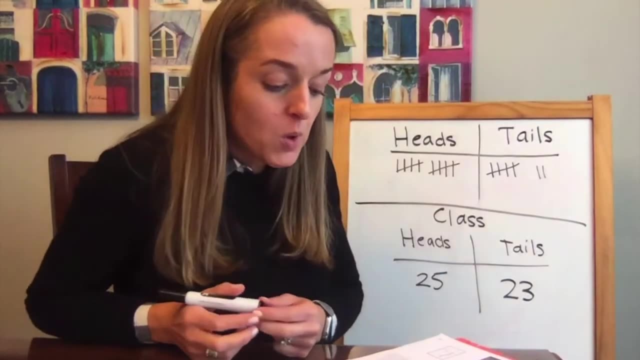 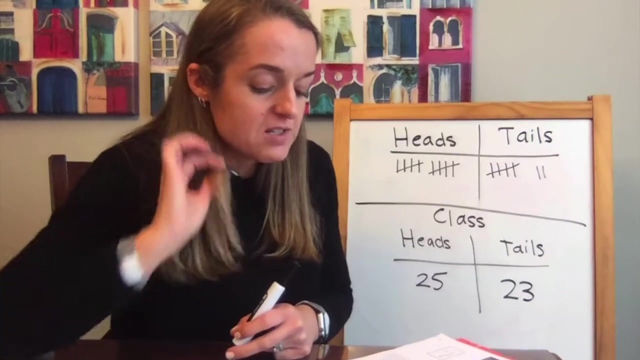 But it's also. it's also outcomes. Sometimes we use words to describe the chance of something happening like impossible, unlikely, possible, even chance, likely or certain. Mathematically, probability is the measure of how likely an outcome is and is expressed. 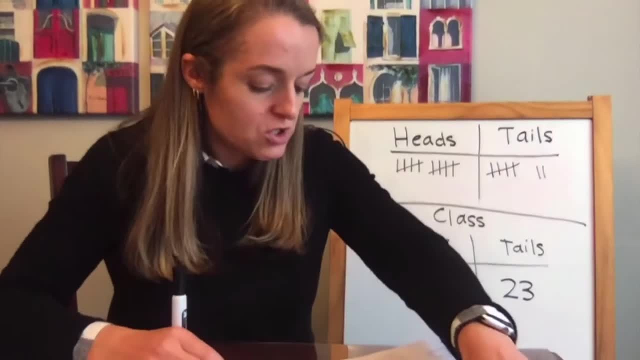 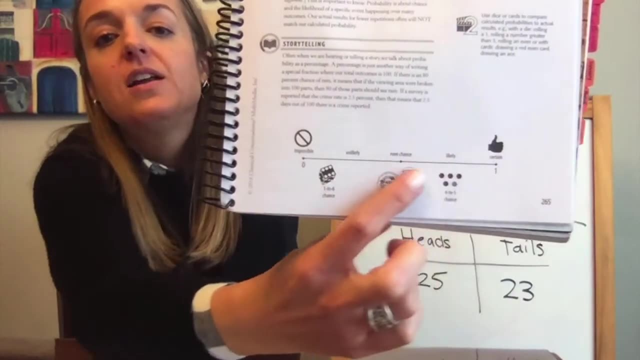 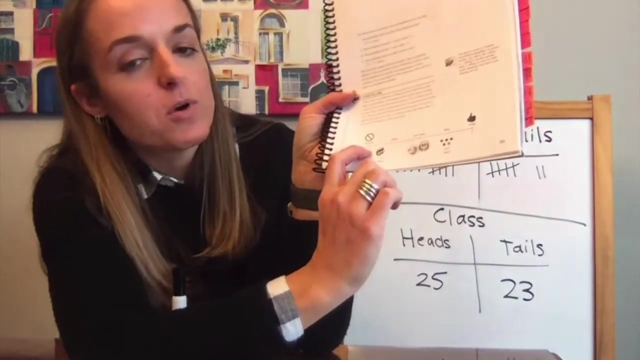 as a number between zero and one. So I want to show you this lovely chart down here at the bottom. If you guys look in your foundations guide and tutors, you guys could draw this on your board. This is a really helpful chart. This chart shows a number zero here at this end and a number one at this end. 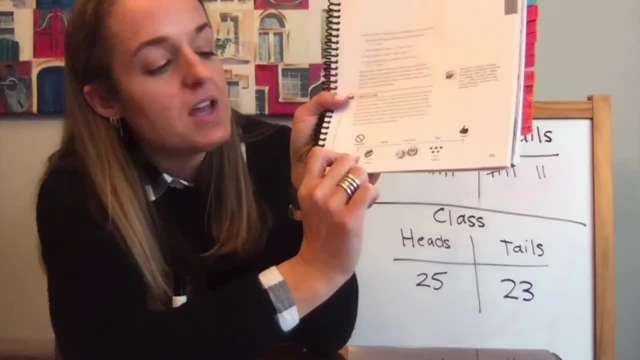 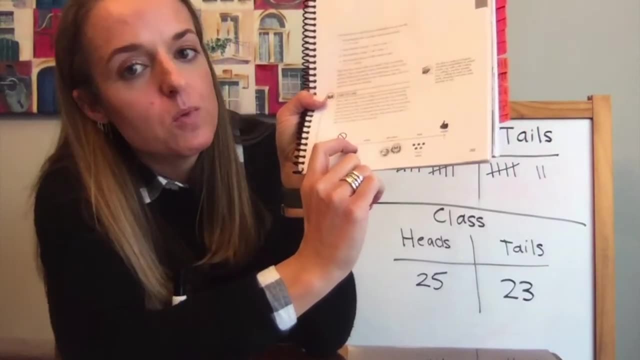 So if we say an event is impossible to happen, so cannot happen, then we're going to say that has a zero chance of happening And then as we go up the line it's going to get more and more likely. So it says impossible, going to unlikely. 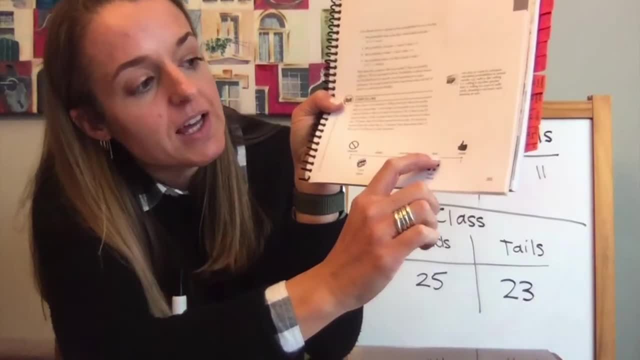 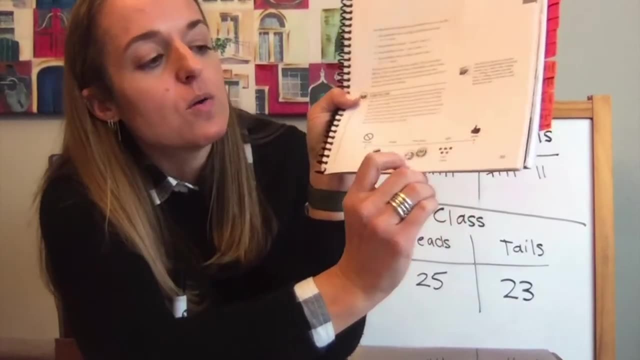 There's an even chance. So it's right in the middle: a likely chance or a certain chance. If it's certain, we know it's going to happen, It's definite, OK. So right here you see a picture of coins with two sides. 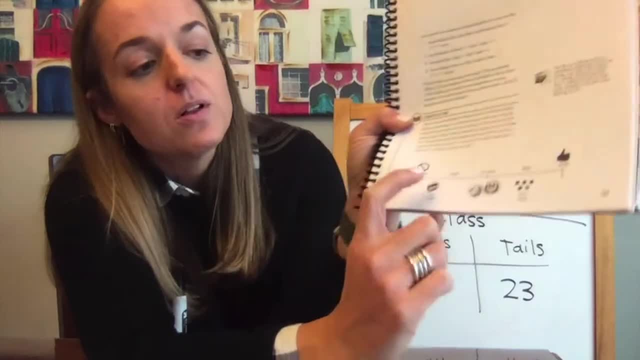 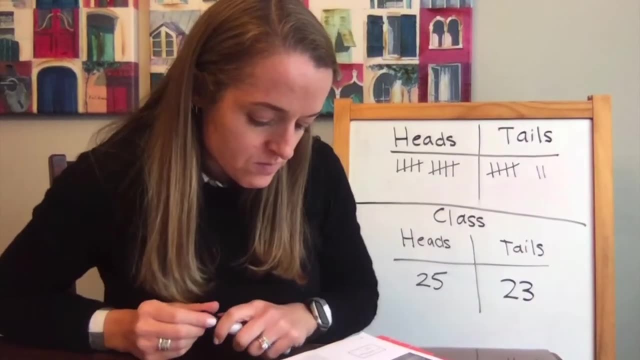 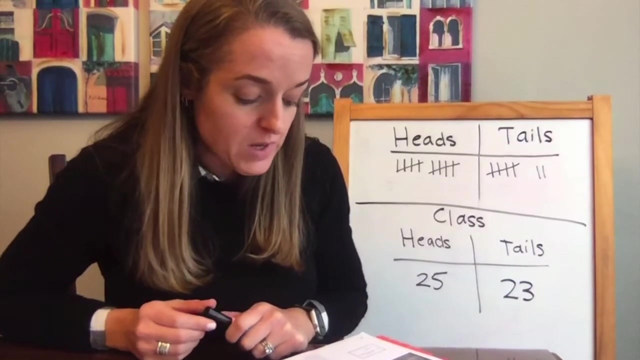 So that is an even chance. So that is squarely in the middle of impossible and certain. So probability is the measure of how likely an outcome is, and is expressed as a number between zero and one. to find the probability of an event, We use a fraction. 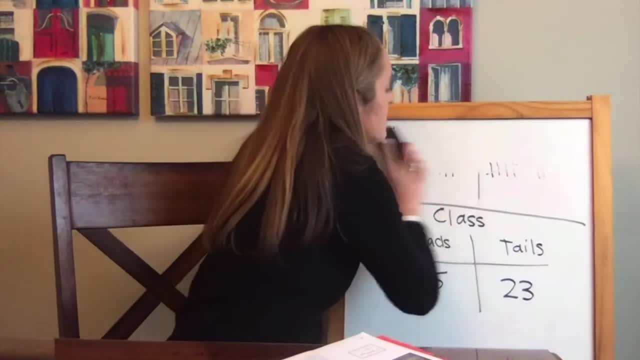 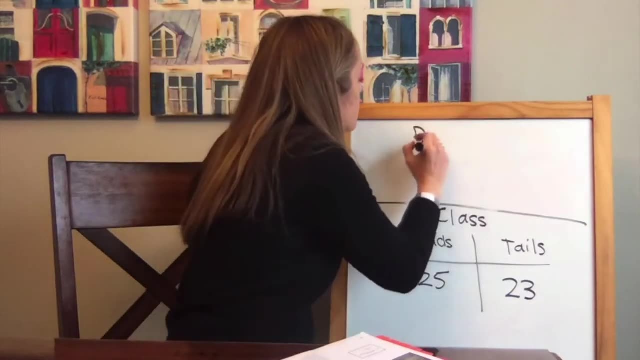 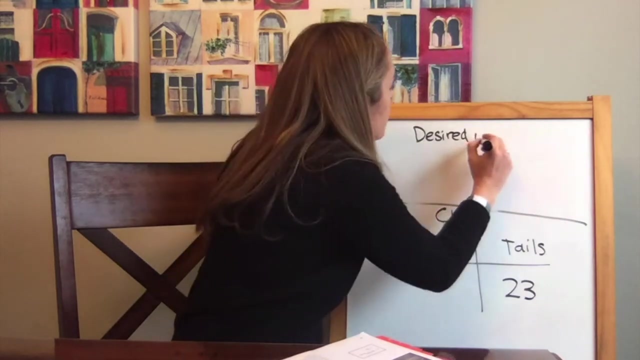 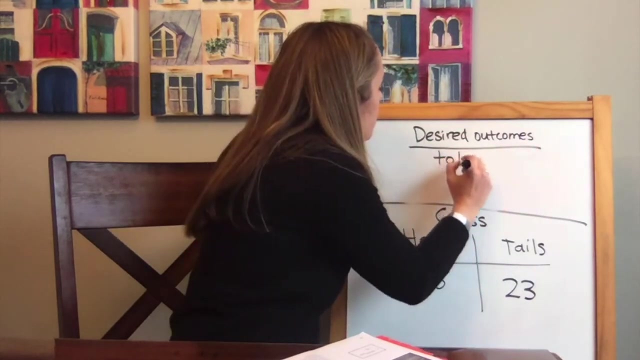 OK, it's a special fraction. I'm going to erase this so I can show you this very special fraction. This fraction is Our desired outcomes On the top, And we're going to draw a line right underneath, and on the bottom is our total. 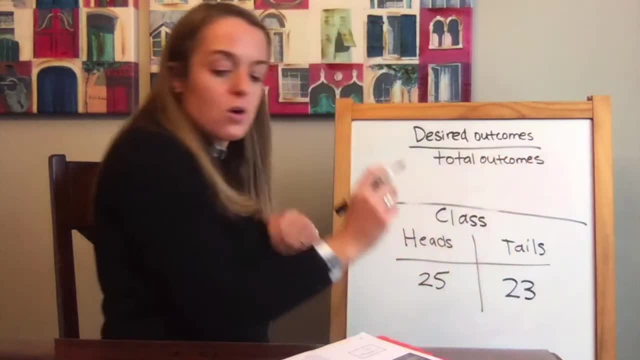 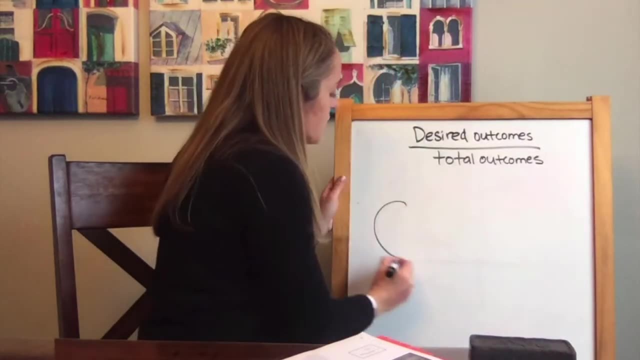 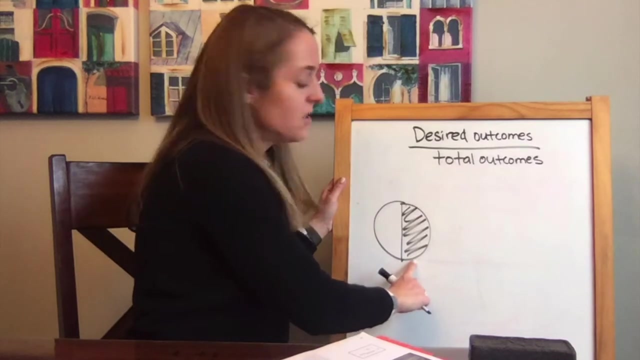 outcomes. Now, if you're old enough to already be learning about fractions in math, then you'll remember that a fraction, if we have this much of a fraction and we wanted to say how much this is as a fraction, we would say that is one piece. 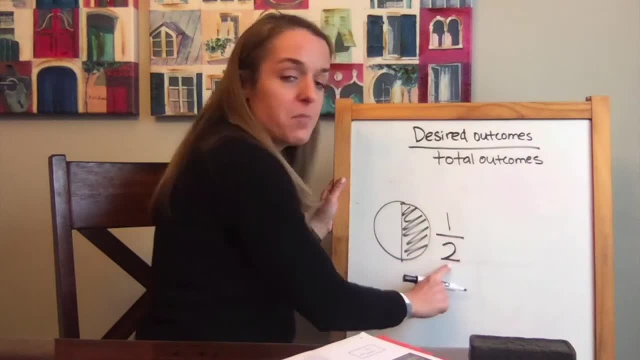 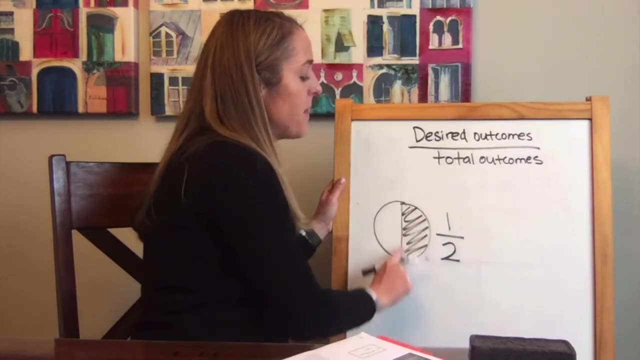 And the whole has two pieces right. So the bottom number tells us how many pieces are in the whole thing And the top number tells us about just the the amount of pieces that we're looking at. So here, with our shaded portion, we're looking at one piece when there are two. 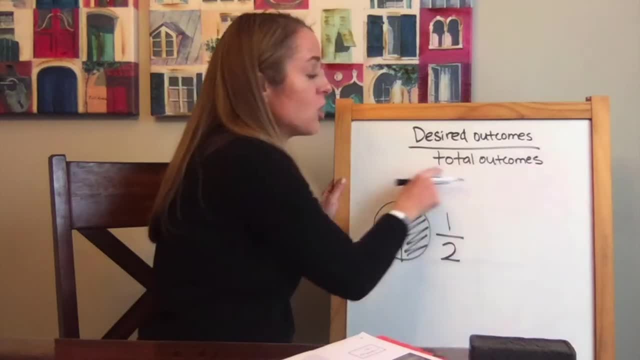 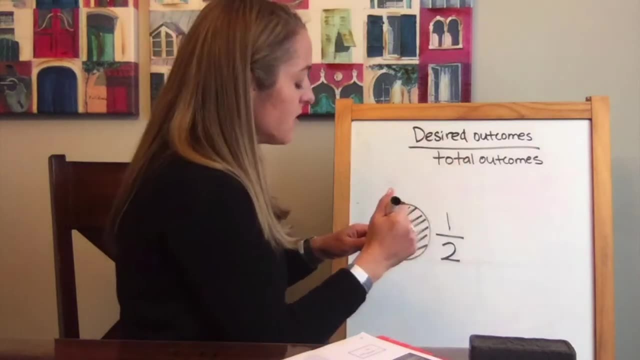 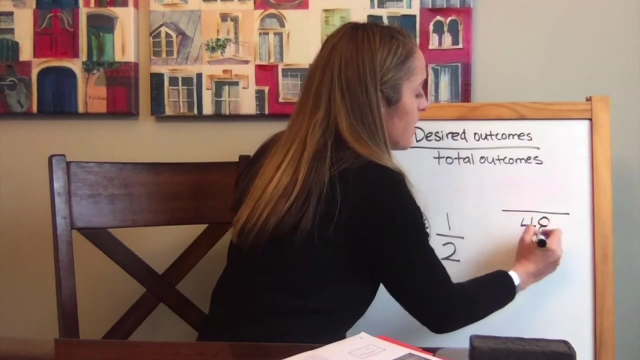 So this is the same kind of thing. The bottom number is going to be our total number of outcomes And the top is our desired number of outcomes. So when we had the heads and tails, when we flipped The coin as a class 48 times, we could say we could say that the probability 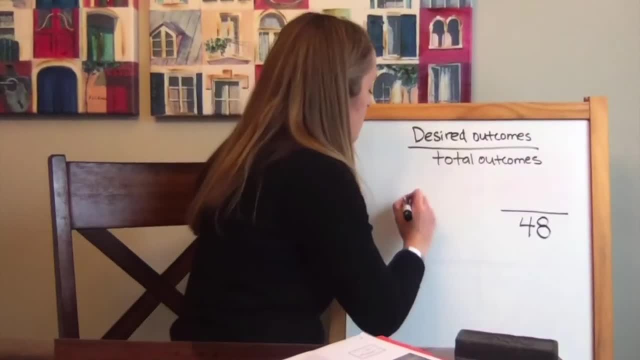 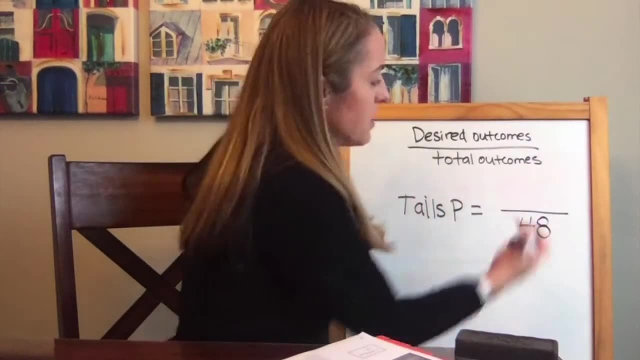 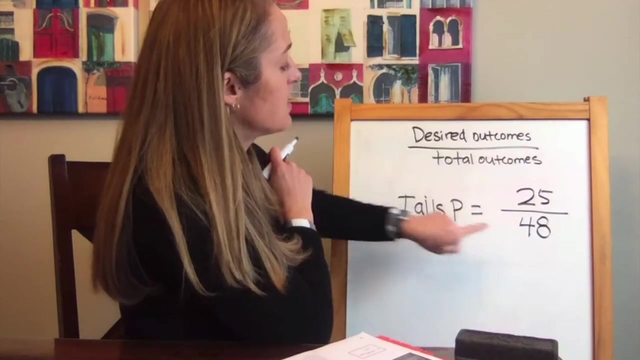 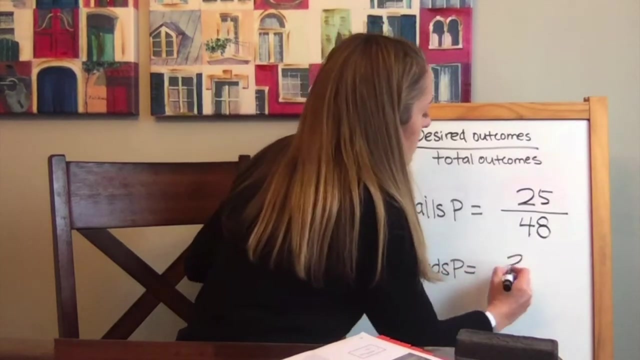 of getting tails. tails probability would equal. I think I already erased it, but let's say it was twenty five. So twenty five times out of forty eight we get tails. and then for heads We I think we had twenty three times out of forty eight. 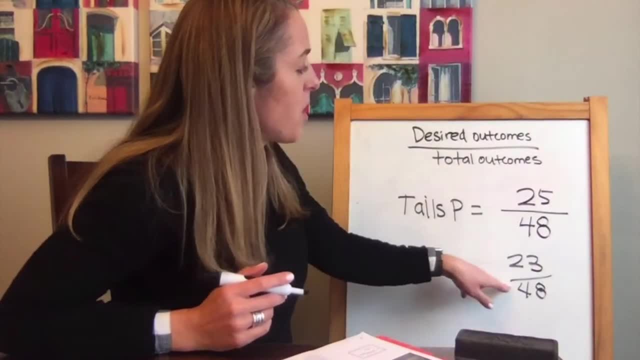 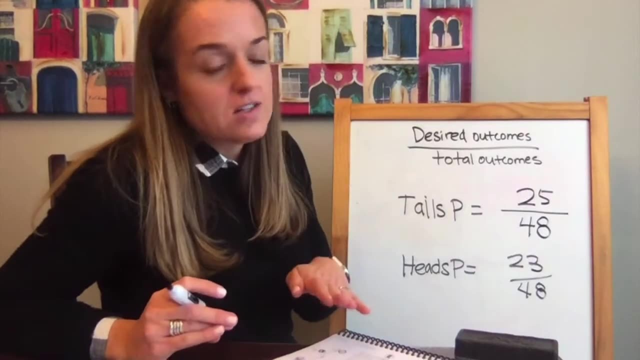 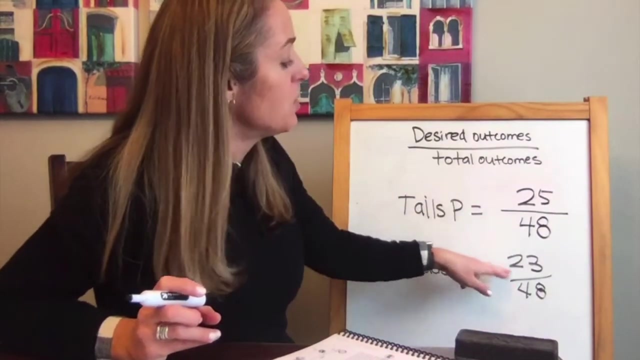 We got heads, So that is our probability. Now, with two choices, we should get a fifty fifty chance, or one over two. If we reduced it for you big kids who know how to reduce fractions, we should get one out of two, which would be half of forty. eight is twenty four. 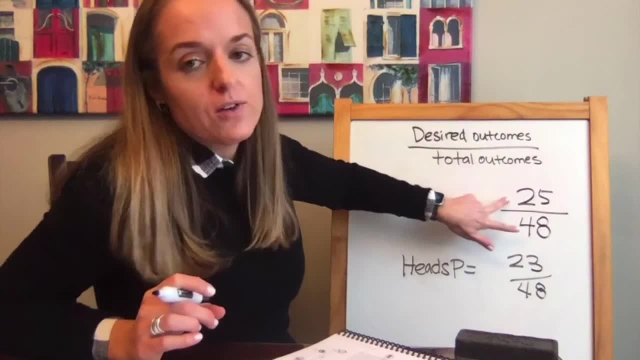 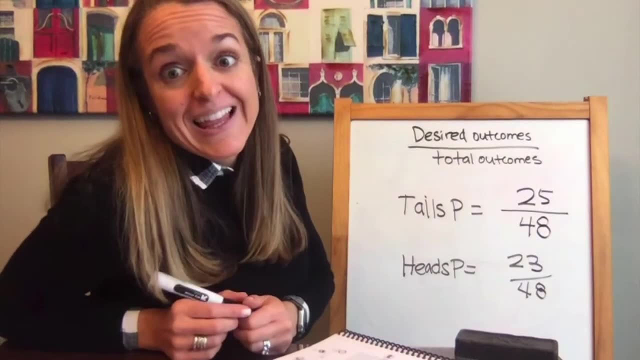 Right, And so we didn't actually get Right on the nose of twenty four. Do you know how we can get closer to twenty four? What would we do to bring this number closer? Do you know We would keep flipping the coin, because the more times you flip, the more. 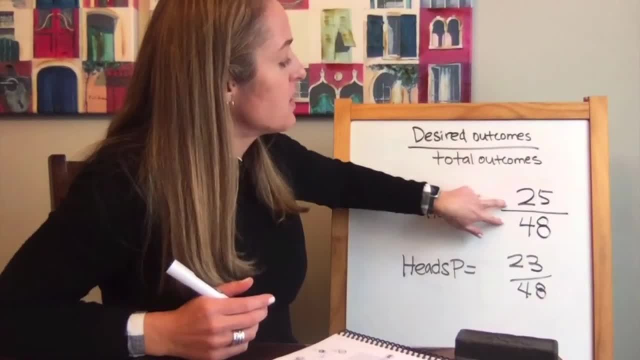 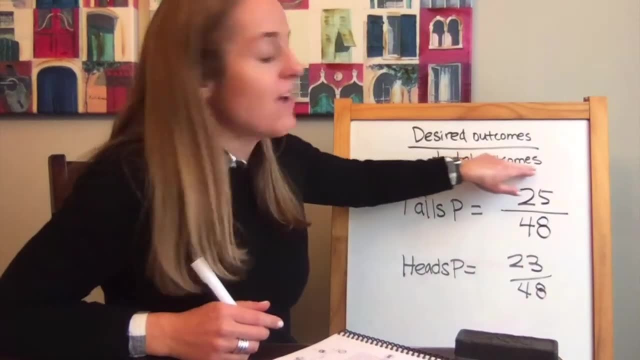 outcomes that you have, the closer this number is going to get to perfectly accurate. So whenever we're talking about probability, we're assuming that many outcomes have happened so that this number is most accurate. So the more times we're going to flip the 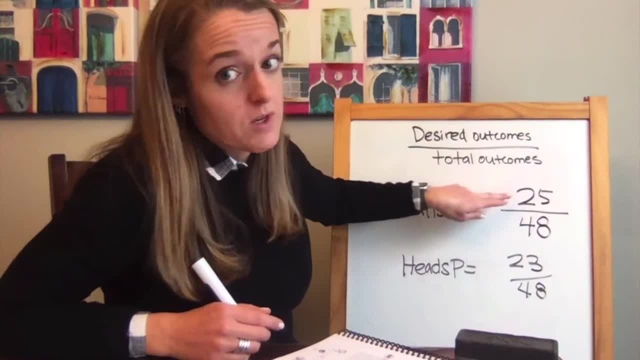 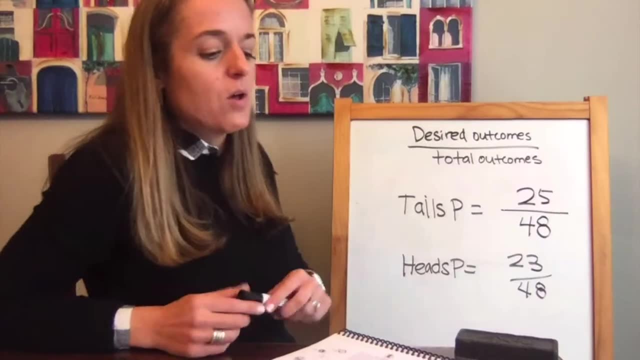 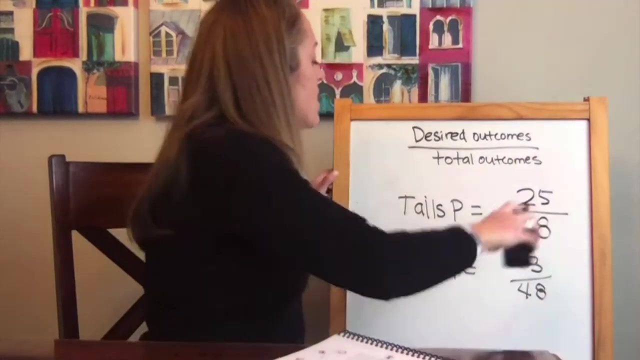 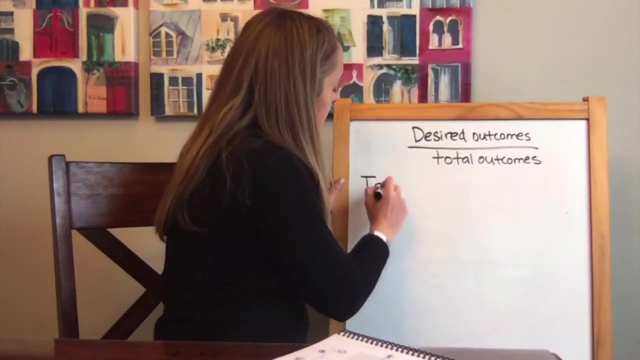 coin, the closer it's going to get to twenty four. Eventually it will get to twenty four solidly, because there are so many flips. So let's talk about the probability that the coin could be flipped. OK, hang on. So, So the probability that it will be tails. 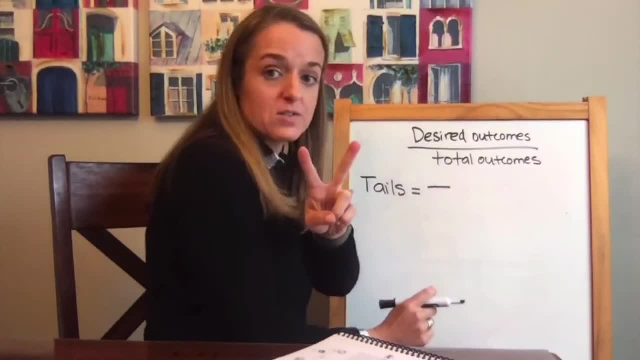 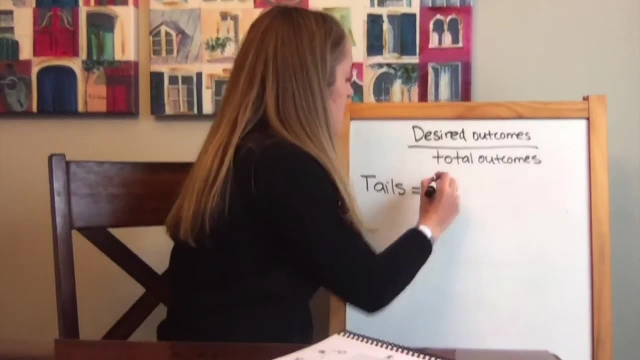 Is There's two choices: right Heads or tails. So the probability that it will be tails is one. There's only one chance it'll be tails out of two chances, because there are two sides And it's heads, Same thing. 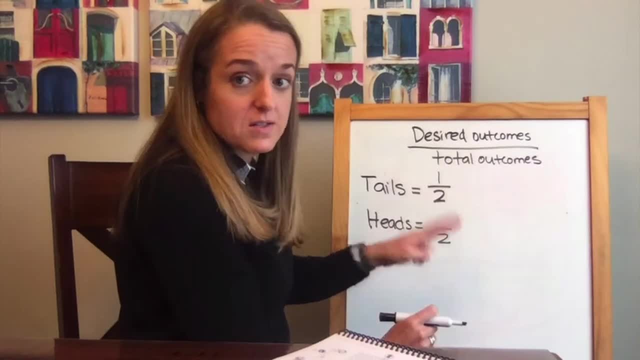 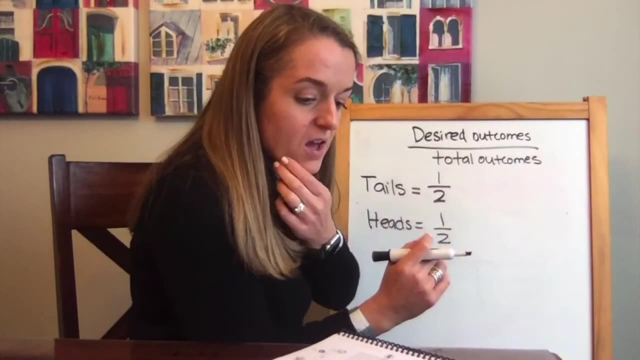 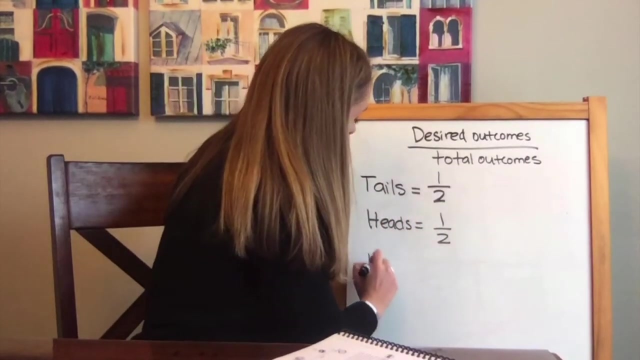 The probability still two chances because you got heads or tails, But the chances it will be heads is just one. What are the chances that it will be both heads and tails will flip the coin And the answer will be heads and tails. What are the chances of that? 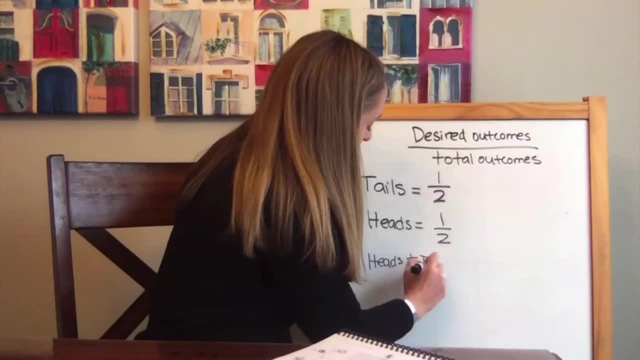 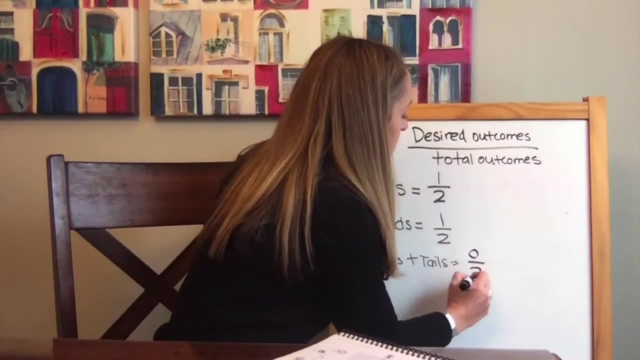 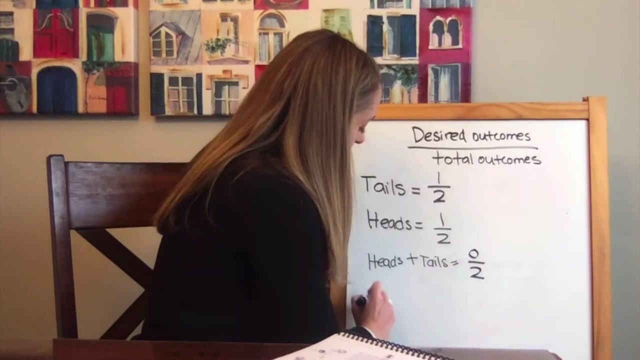 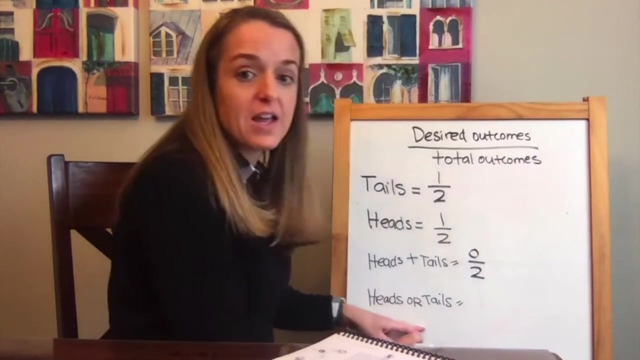 I'm going to write this down: heads and tails. Can that happen? No, So that is zero over two. That is impossible. You cannot get heads and tails at the same time. What are the chances of getting either heads or tails? So this time I'm saying there are two choices. 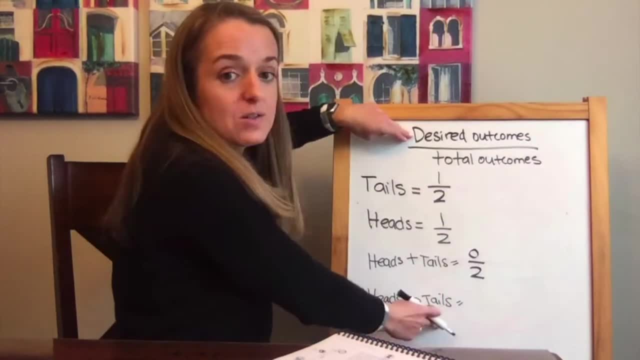 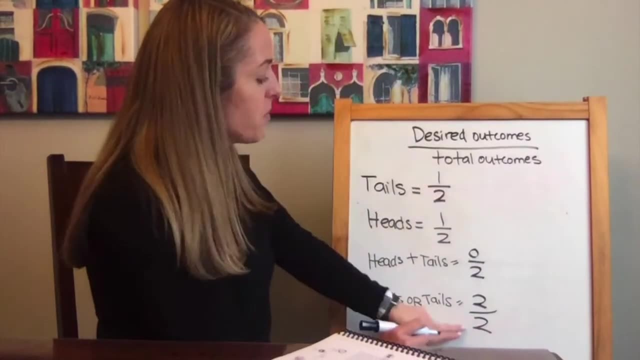 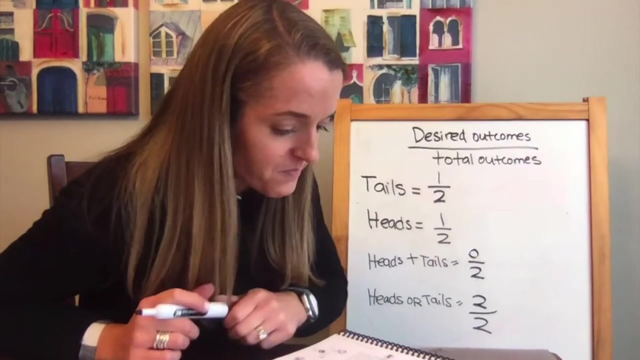 There are two desired outcomes. I can either get heads or I can get tails. So with two desired outcomes and only two total outcomes, my fraction, my probability, is two over two. That means 100 percent of the time I will get either heads or tails. 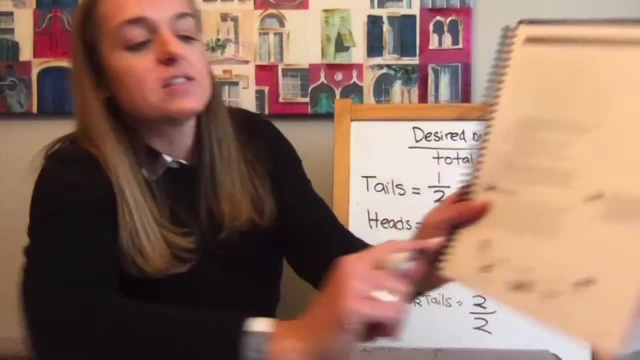 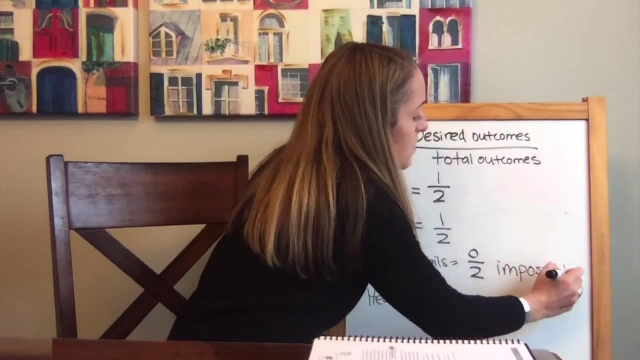 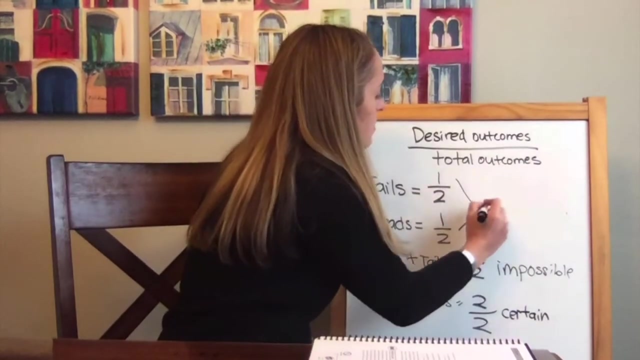 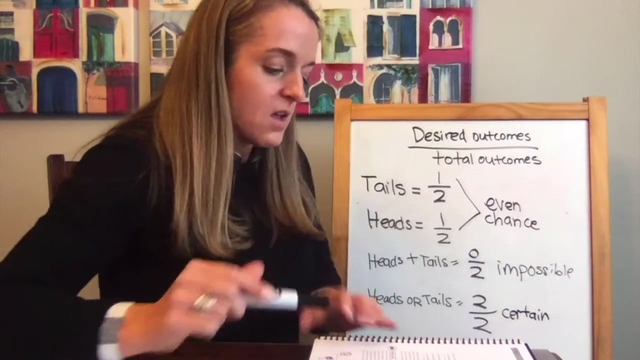 I will always get that. So if we look at our slider here again, this one is impossible, This one is certain. We are certain to get one or the other, And these two we have an even chance. So if you want to see for yourself if we keep flipping a coin, if you have more, 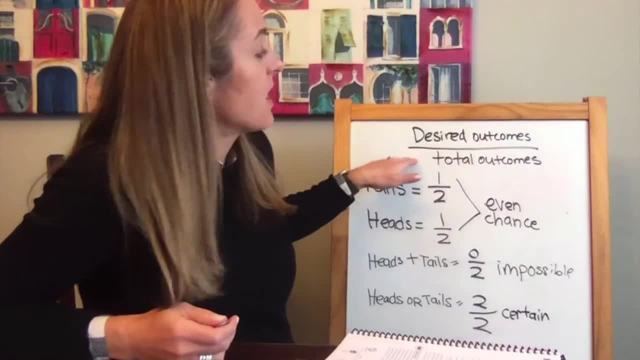 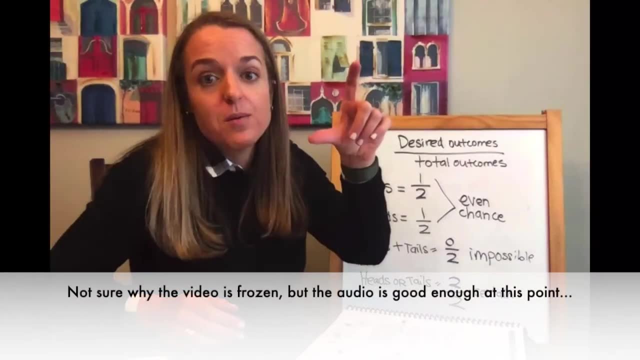 time in class and you want to see we can keep flipping a coin and we can keep adding to our partner, tally and keep adding to the class tally and see how that number gets closer and closer, and closer to actually one over two or twenty, four over forty.